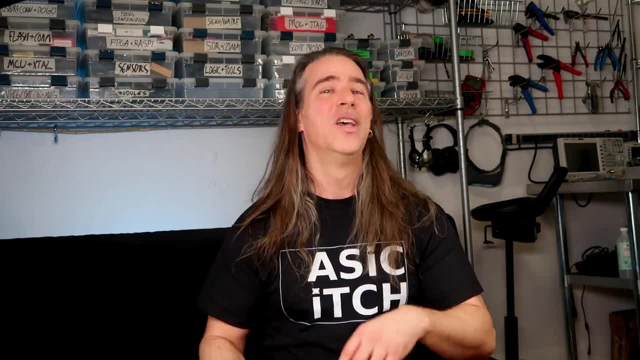 and I've already made some interesting discoveries about simulation with NG-SPICE, using layout tools and more. I'll be posting details about those finds and everything else I encounter here, and I'll be posting more details about what's going on in the future. 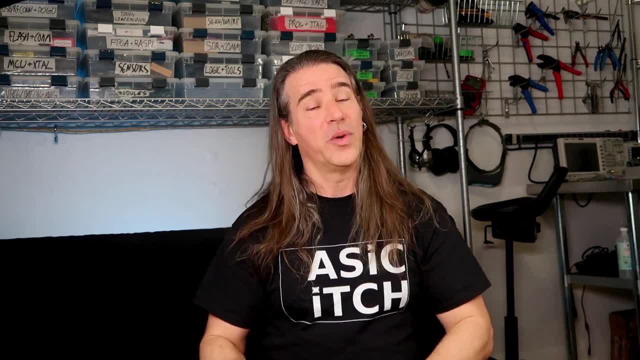 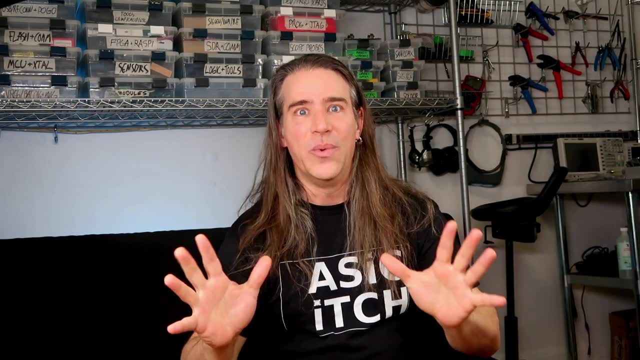 And title the content with the keyword ASIC or something, so you can catch them when they come out. For right now I want to show you something pretty sweet that's a quick intro and lets you play without installing anything at all- The Silly Whiz. There's a step-by-step tutorial. 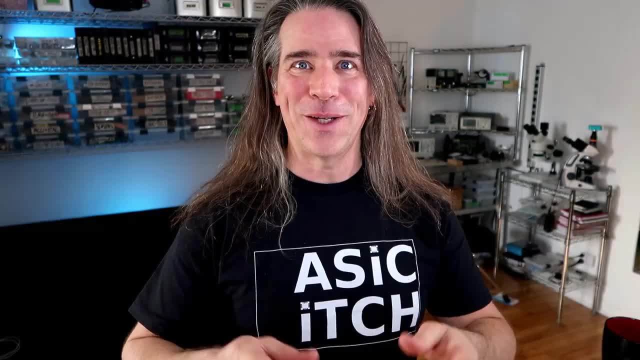 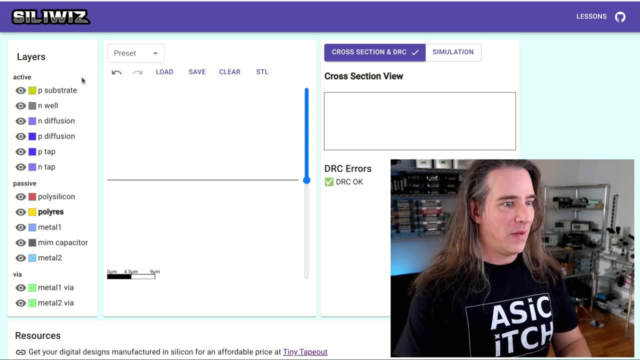 that walks you through everything, but let's do a couple of quick examples. All right, check this out. So this is the Silly Whiz interface, and it's pretty much more whiz than it is silly, as you'll see soon. I find it pretty cool. 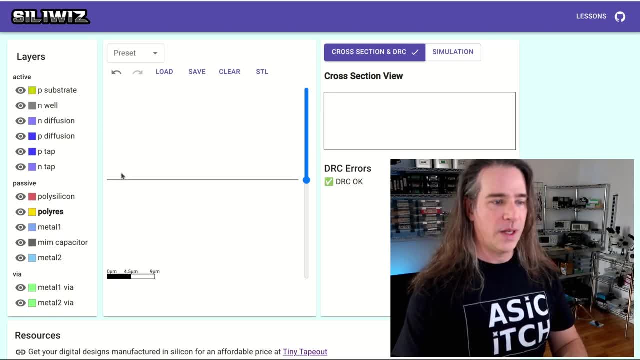 So let's start with something really easy. I've got this poly res material here selected and I'm going to draw something. All you do is basically go into the canvas and draw a little square and that's it, your rectangle. And what have I made? Well, it's a resistor, Not very useful. 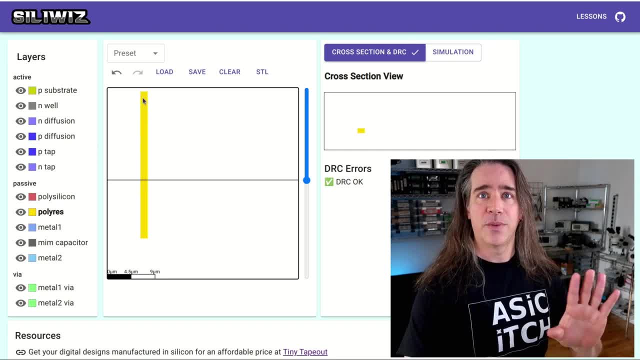 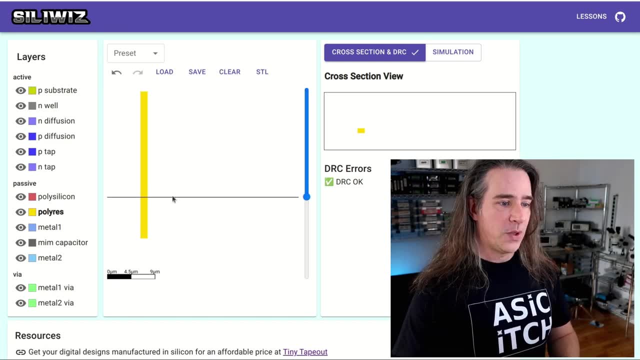 right now, but that's all it takes. This is semiconductor. I've got a little strip. It's a resistor- Cool. Now you can actually see the cross-section view, which is not very interesting right now. It's right here, So that's cool. Now let's do something a little more interesting. 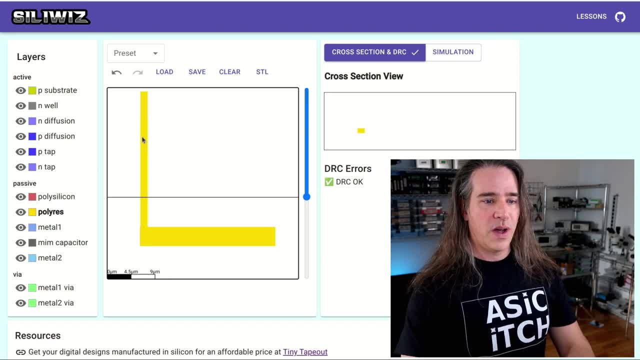 Let's go and make a voltage divider. So now I've got well, what will be two resistors? It's just one big strip, It's more like a potentiometer actually. So let's see, I'm going to put some vias here, because we need to connect this to the outside world. 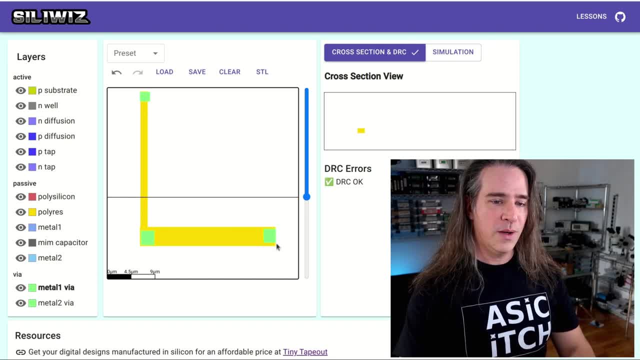 So I'm going to put one here and one here and one here, And if you look at the cross-section there, you can see they're building on top. So what we're trying to do is get to metal one so that we can actually connect things to electric things. So I'm going to put three vias here. 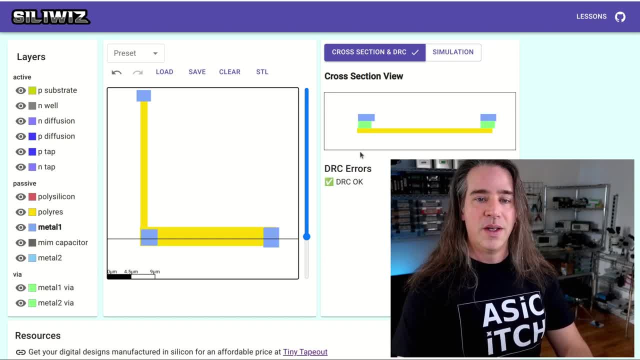 And, as you can see, these squares. Okay. So now I've got a little sandwich, not super duper useful. Now I'm going to tie them to something, And some of the magic here depends on naming things correctly. So basically, what you want to do is call one of them, set the. 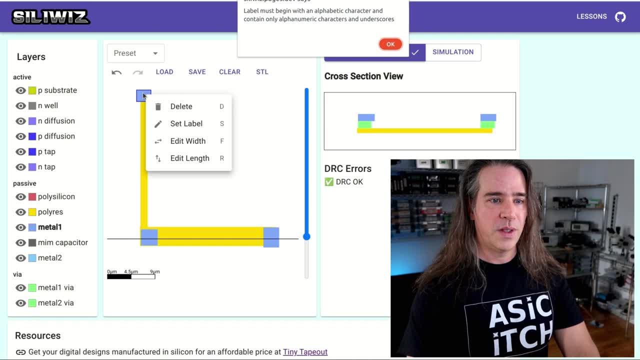 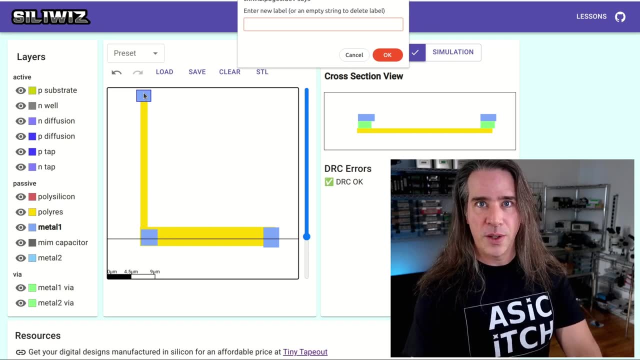 label to in? What label must be: Yes, Yes, Sorry about that. Sorry, Mr Wizard. Okay, Now I'm going to set a label to one of these magical keywords, which is in. I'm going to set this one. 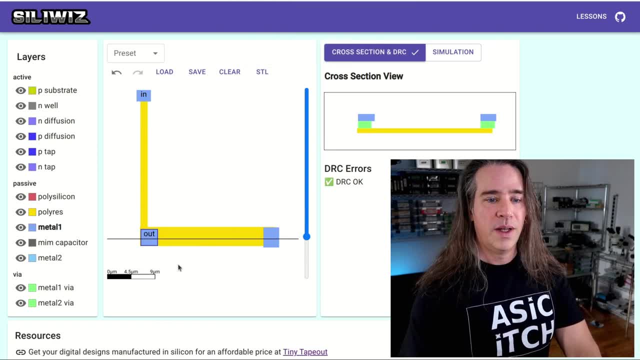 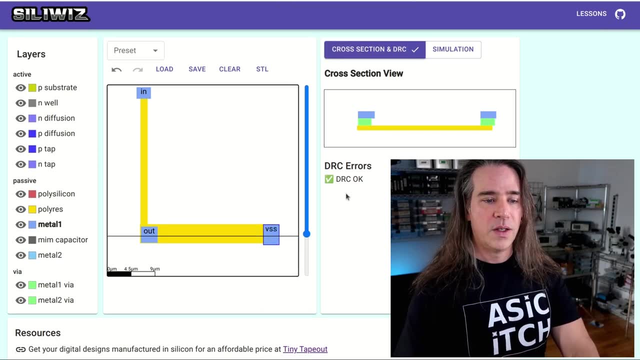 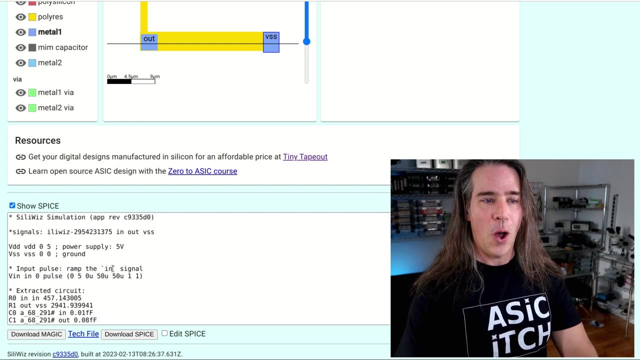 which is in the middle of our divider here to out, And then this resistor, we'll go to ground which by convention here is VSS. Okay, Oh, look at that. So now what happens is that this spice is being generated here and we have some resistors detected. Okay, So we can look. 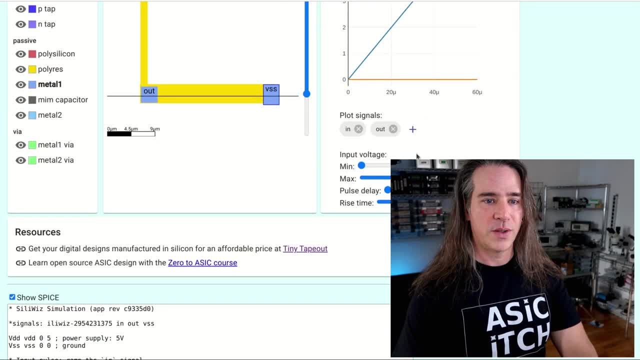 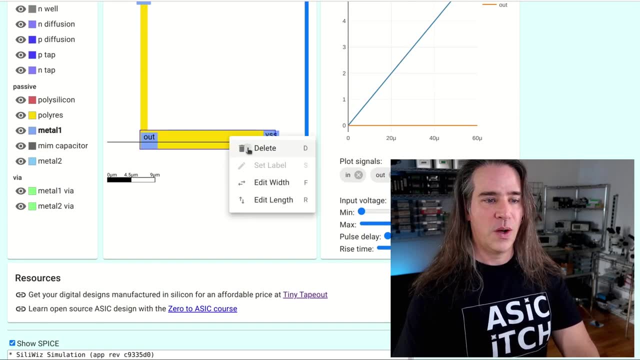 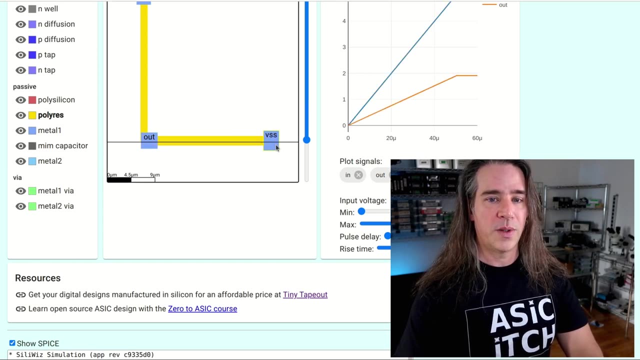 at the simulation and, well, nothing very interesting is happening at this stage. Why is that? I think that this resistor is just too small, So the value is small because it is fat and it's letting everybody through like there's no tomorrow. So here we go, I'm going to try that. 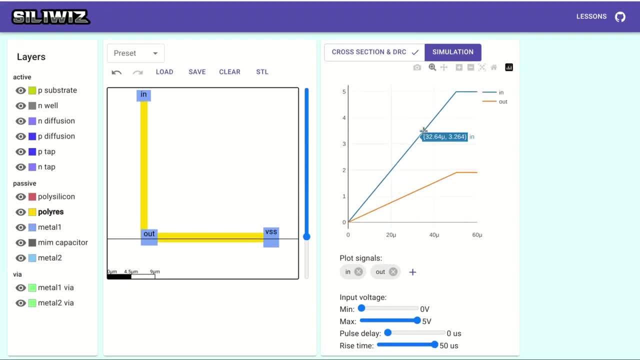 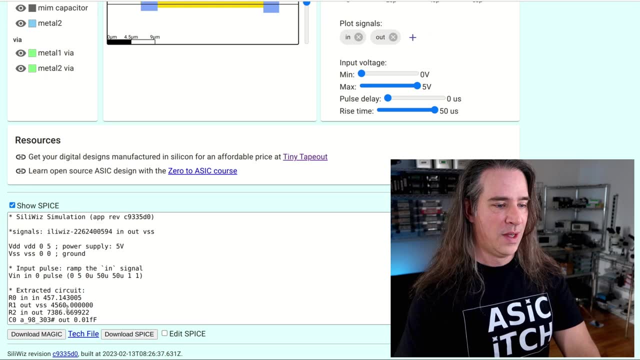 Well, suddenly we have a voltage divider action here. So at four volts we're a little bit under two, which means we're a little less than half the resistance in that one. So let's see what that says. So we've got a little less. Yeah, So seven K and four and a half K. So I'm going to try to. 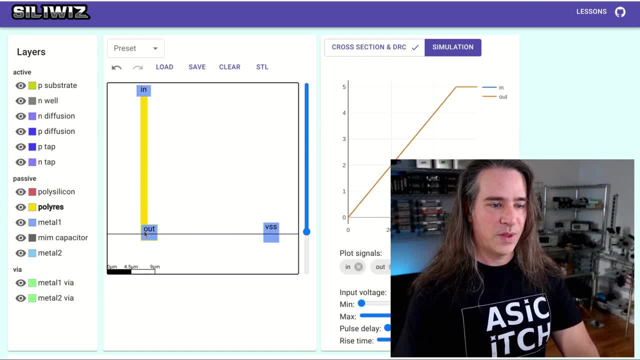 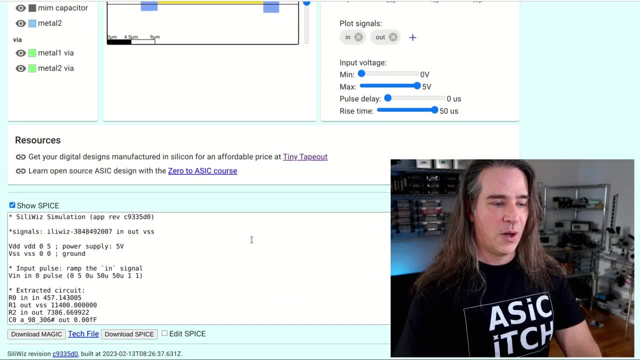 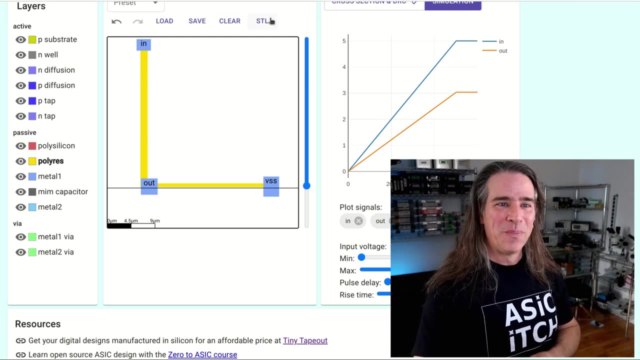 get it to a half. Uh, it's shorter, so it's got less resistance in general, So I'm going to make it a lot thinner. Let's try this. Ooh, I think we're getting close. So 11 K, eight K, whatever voltage divider. Now I promised a MOSFET, So let's do that. 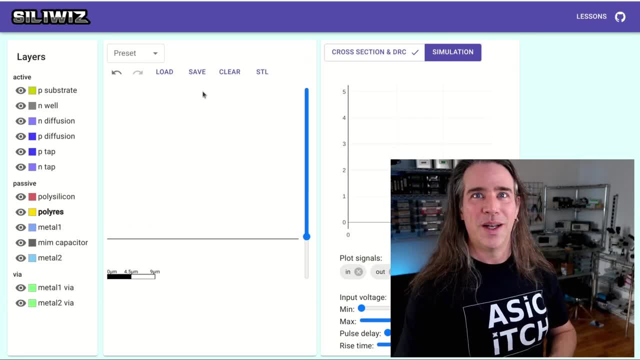 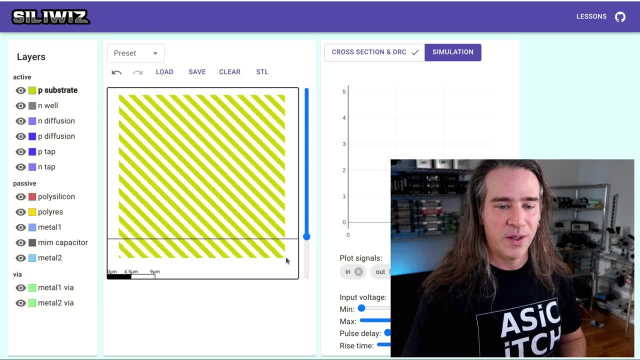 I'm going to clear this out a little more complicated, but more interesting as well. So, uh, first of all, everything is built on a single substrate, and this is a P type material doped with holes. I'm a physicist first and I always found the traveling whole thing a little. 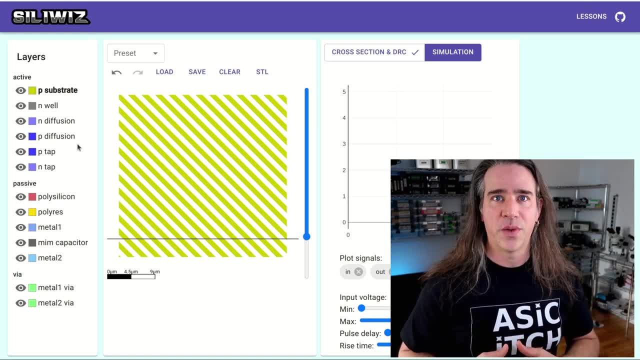 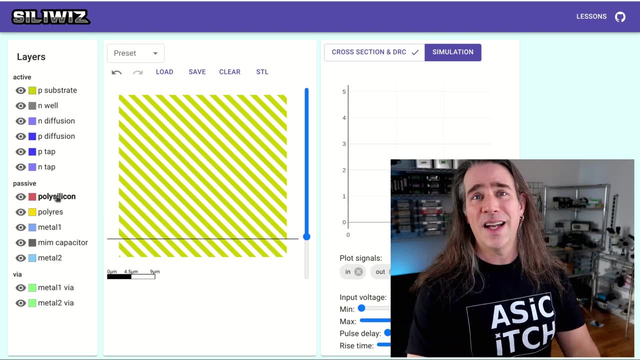 bit annoying, Uh, but uh, it's actually a useful tool for thinking anyway. So we've got this P substrate and we're going to try to get it to a half volt. Okay, So we've got this P substrate and what we're going to need is to create our MOSFET. So I'm going to choose this polysilicon, which is: 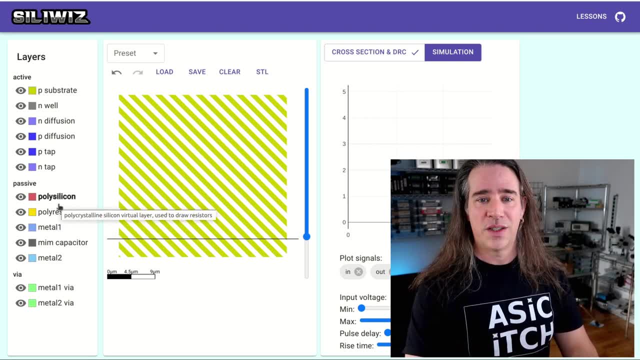 actually exactly the same uh material as this poly res. It's just that for that uh spice magic down there to work, uh, we need to kind of separate them out in different layers. So, um, polysilicon is going to be our gate and we're just going to make a fat gate here and under that gate. 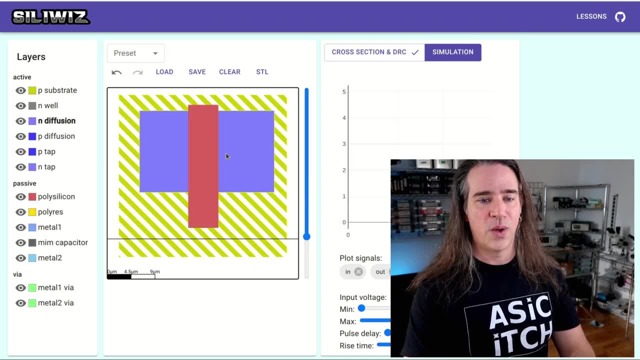 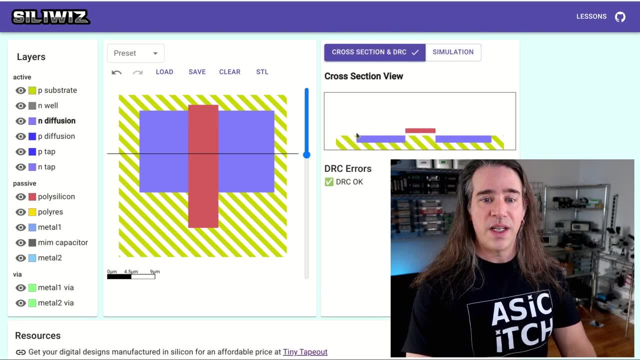 and diffusion. So that's another thing under that gate. I said you can do them in any order. but uh, the process is the process. So here we look at the cross. So here we look at the cross section, We can see the end. diffusion is actually diffused inside to the P. So this P stuff becomes. 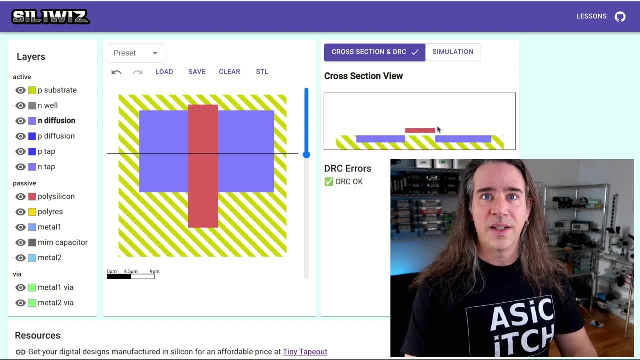 uh N stuff and the gate is on top and it's actually masking that part of the process, So the diffusion doesn't make it through. So this middle part stays uh P. So what do we have here? We've got N and some gate uh insulated here from the rest, and another N and spices actually detected. 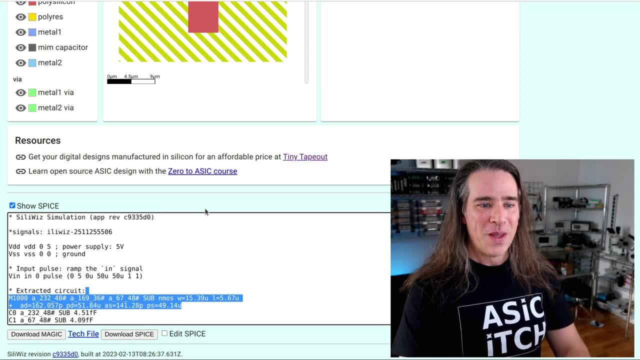 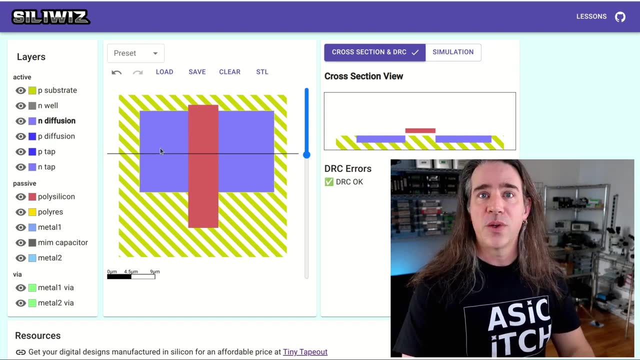 an NMOS. That's pretty cool. Okay, So we have a MOSFET here, but we don't- uh, we can't, actually use it because we need to connect it to the world. Uh, we need our drain source in the gate and we. 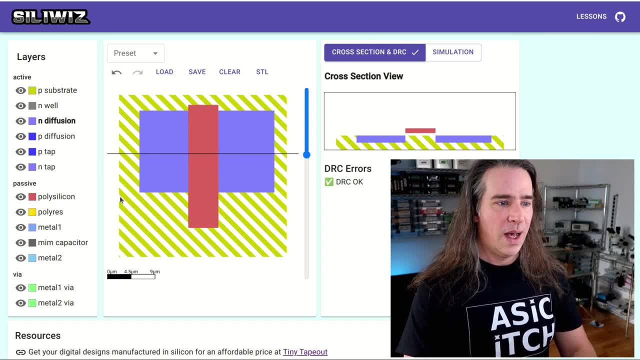 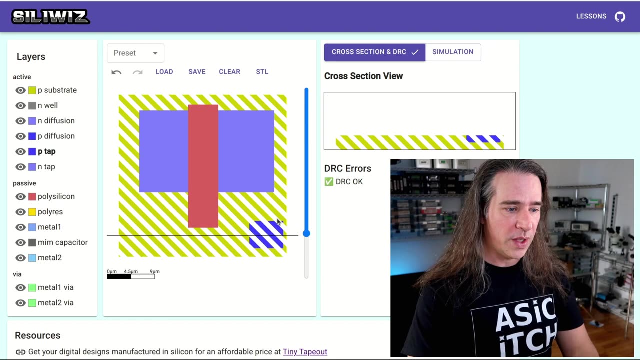 need a body connection. So, for the body connection, this is already P, uh, but apparently we need to increase its penis, Um, so do you do that with a P tab here, which is another thing like the N, except that instead of making it N-ish, it's uh, more, more holes. So there you go. Now all we do. 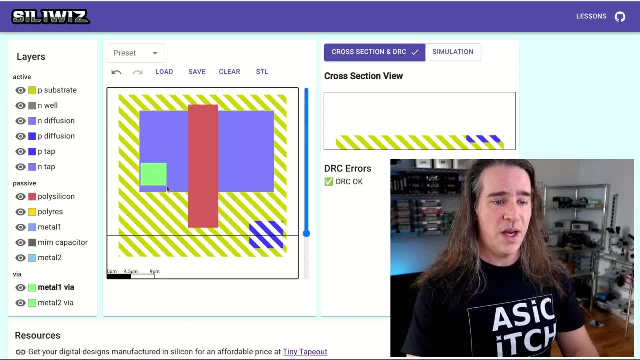 is like: before we stick some metal, bet Kaliris on everything. So I'm going to stick one here and I'm going to stick one here, That'll be our gate. and here now, which is the drain, which is the source. This thing is perfectly symmetric, which I find very interesting. Uh, so you get to choose. So I'm going to put some metal, metal, metal, metal, and it's pretty forgiving. Look, I'm making these big fat squares everywhere and it just doesn't care. So look at that. My stack up isn't super pretty, but it's going to work. So I'm going to put some metal, metal, metal, metal, and I'm not going to just use forущ, but pretty, pretty gentle bit. 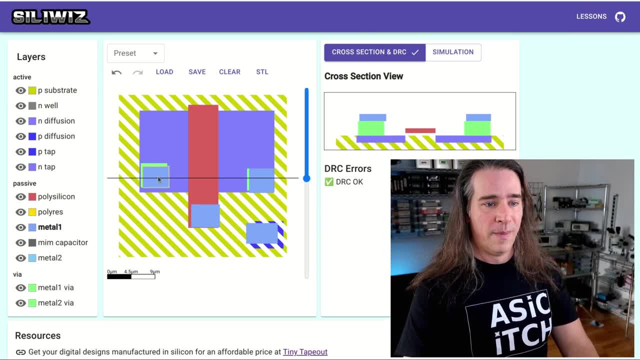 just look into it. So look at that. My stack up isn't super pretty but it's going to work. So you can see in my stack up People always want a. So let's call this, let's tie this to ground here. 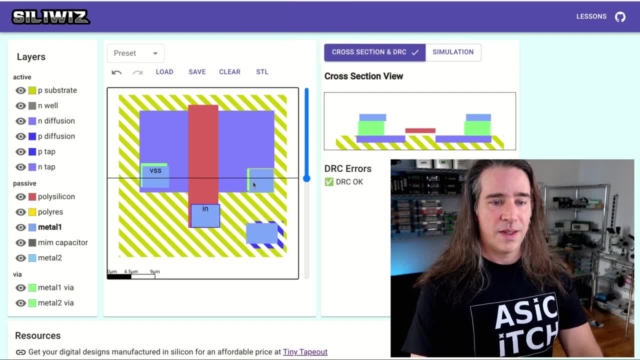 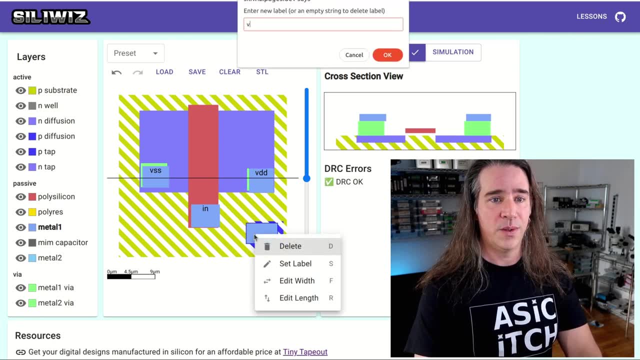 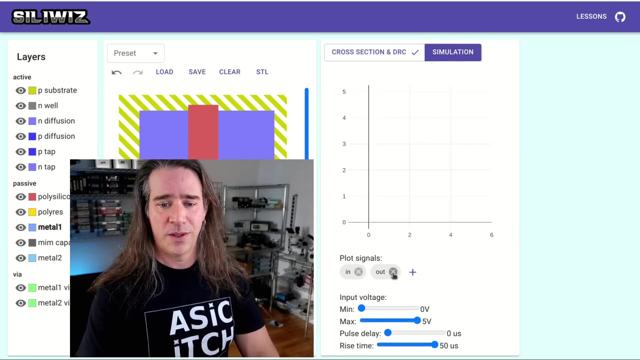 Let's say: this is the input, Let's tie this to VDD straight up And finally, this one is our body, so we'll set it to ground. Okay, now what's the simulation say? The simulation says no thing. I'm so unhappy because what the hell are you talking about? 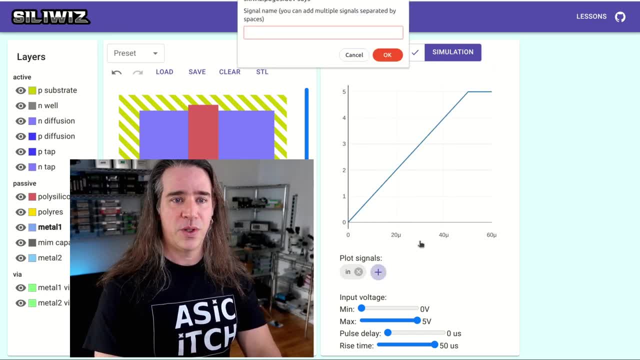 Out. Well, okay, out doesn't exist, but let's put something. This is spice stuff, so we can do spice things. Now I'm just going to scale the current through VDD there and see what happens. Well, this looks diode-y, transistor-y.